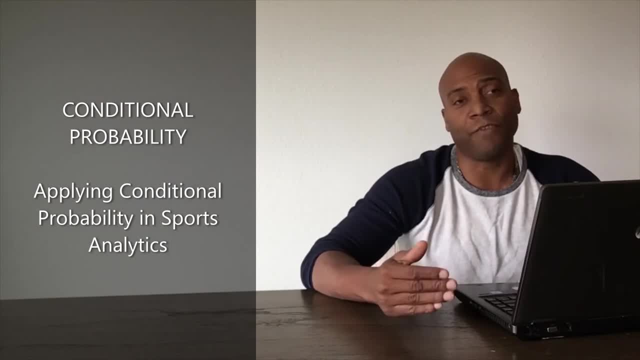 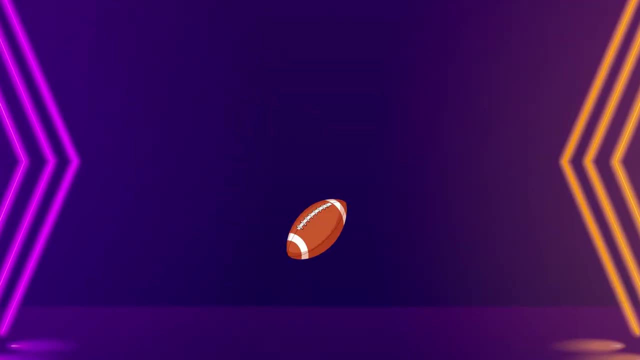 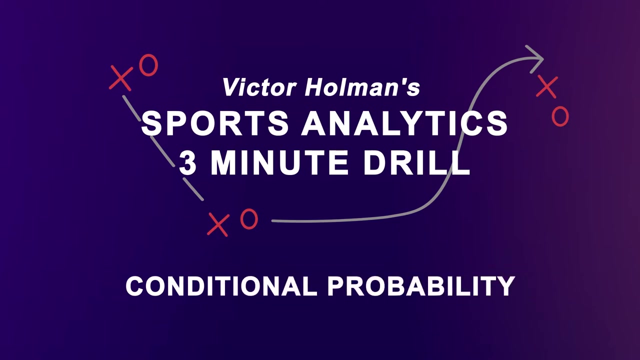 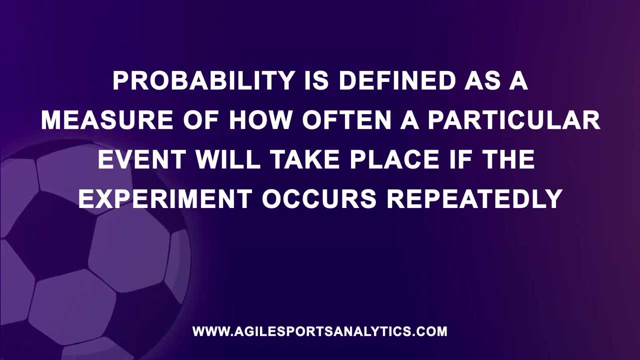 And remember, if you find this video informative, please like the video or subscribe to my channel. So let's begin. Probability is defined as a measure of how often a particular event will take place if the experiment occurs repeatedly. Probability ranges from 0 to 1.. 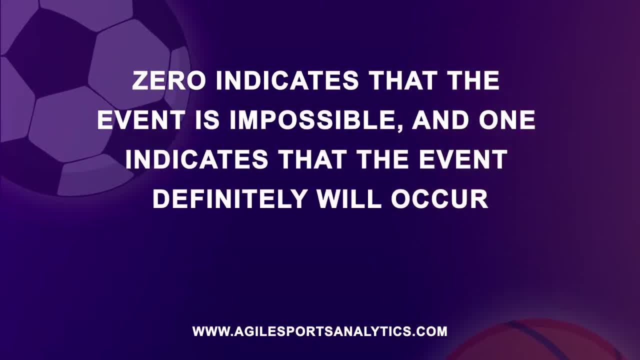 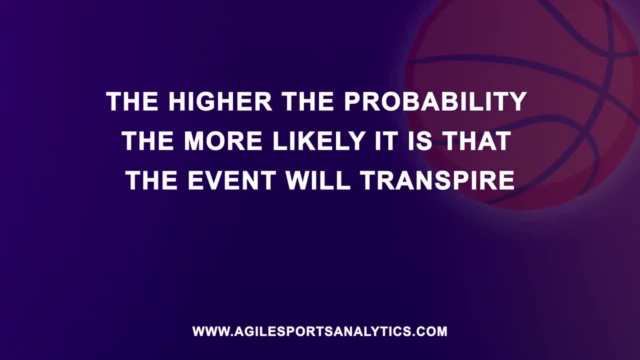 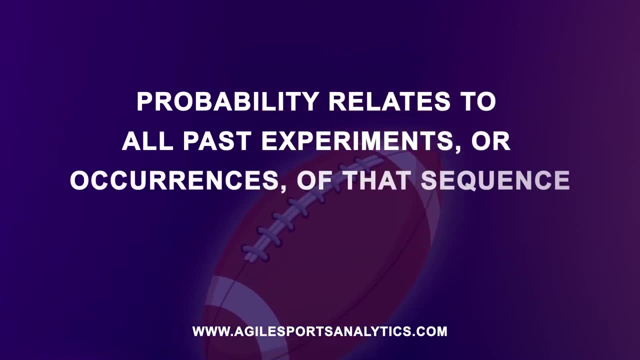 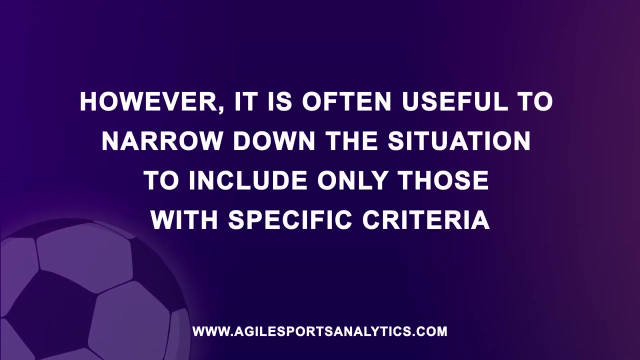 0 indicates that the event is impossible and 1 indicates that the event definitely will occur. The higher the probability, the more likely it is that the event will transpire. Applying conditional probability to sports analytics, Probability relates to all past experiences or occurrences of that sequence. However, it is often useful to narrow down the situation to include only those with specific criteria. 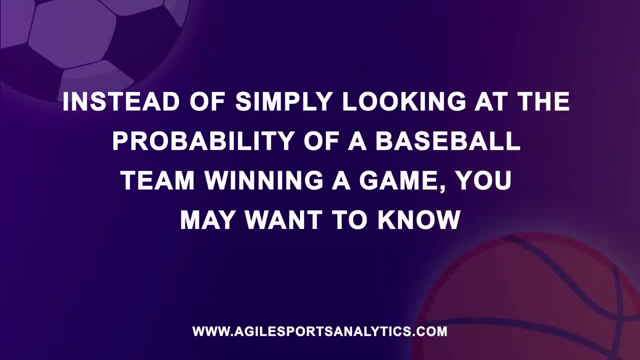 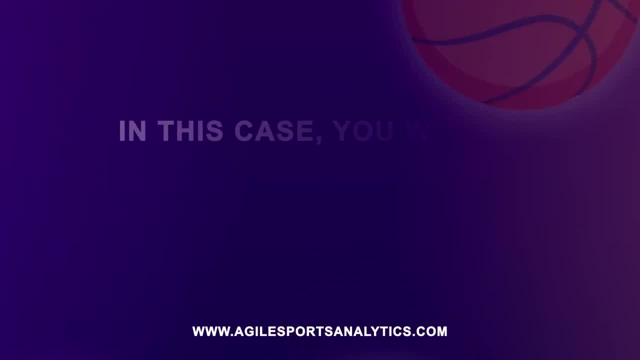 Instead of simply looking at the probability of a baseball team winning a game, you may want to know the probability of the New York Yankees winning when Aaron Judge hits a home run. In this case, you would use conditional probability. Conditional probability is a measure of the probability of a team winning a game. 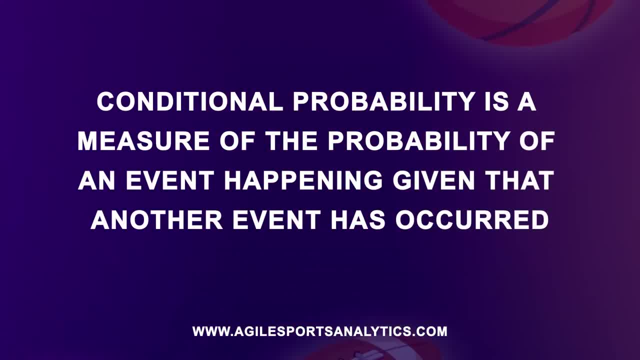 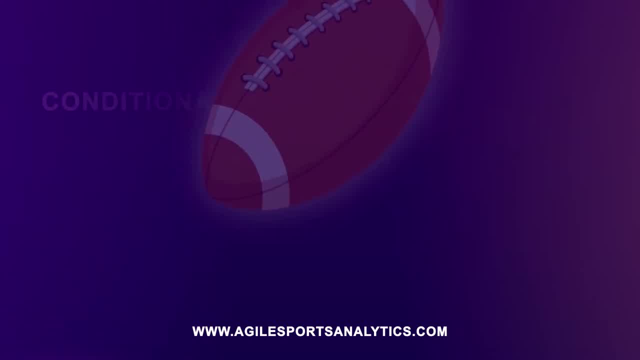 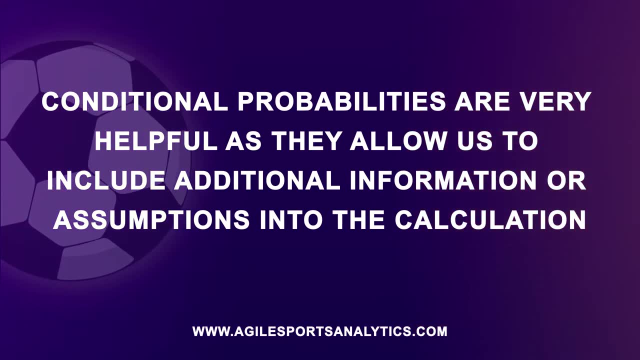 Conditional probability is a measure of the probability of an event happening given that another event has occurred. Conditional probability allows us to add extra conditions to the scenario we want to explore. Conditional probabilities are very helpful as they allow us to include additional information or assumptions into the calculation. 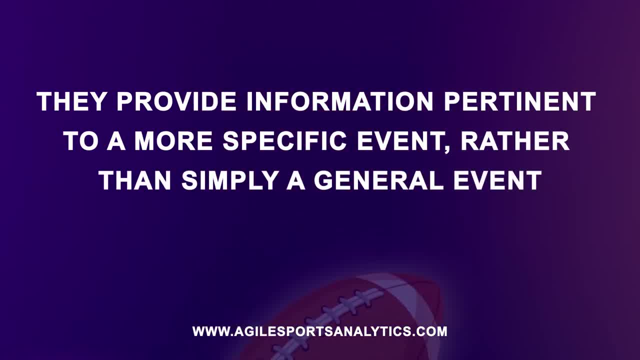